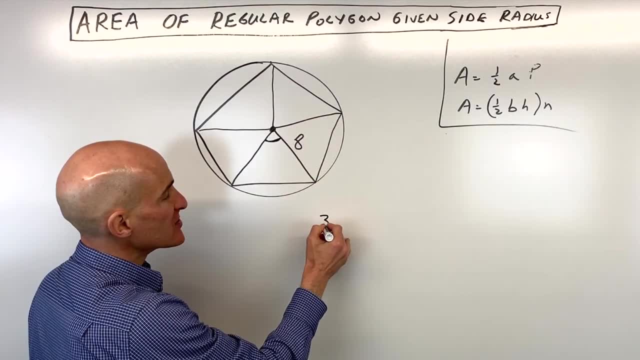 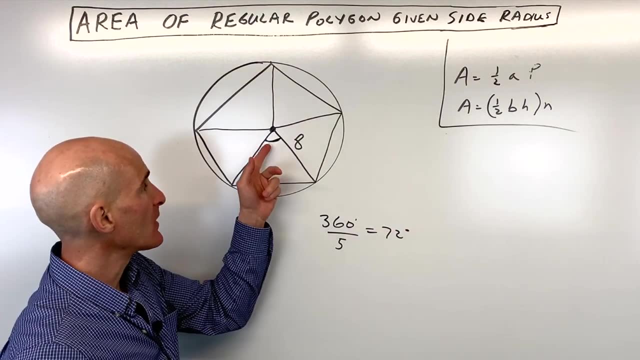 want to find that central angle. And we know in a circle there's 360 degrees. so if we divide that by five, since there's five of them, that's going to give us a central angle of 72 degrees, right. But then if we drop an altitude here, which this is called the apothem- okay, it's also the height. 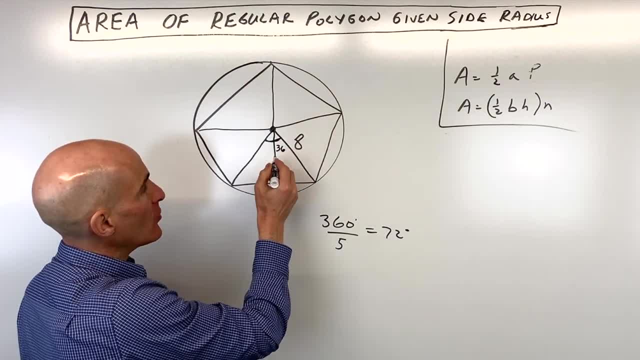 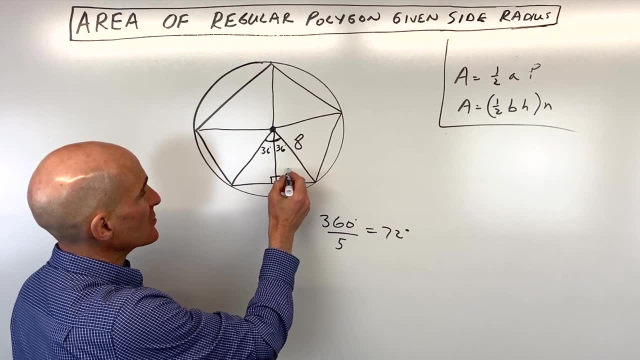 of this triangle here. it's going to split that 72 degree angle into 36 and 36.. And we know that the hypotenuse here is the radius. okay, across from the right angle that's eight. But how do we find out the area of the pentagon? Well, we want to find out the area of the pentagon, So let's. 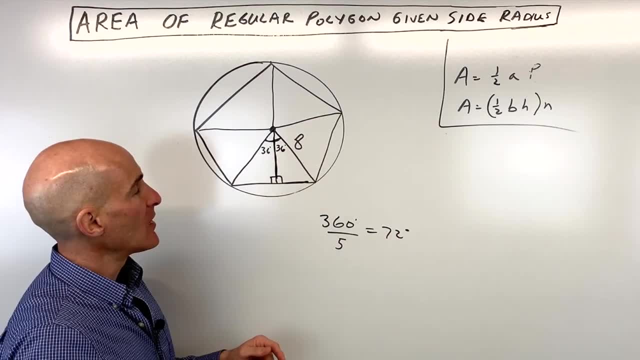 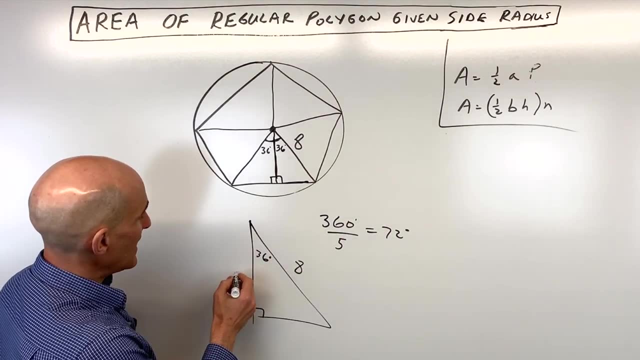 find out this side length and this side length. Well, let's go ahead and make this triangle a little bit larger so we can see it. So we have 36 degrees, let's call this eight, let's call this a for apothem and let's call this x for the side length. So we're going to use a little bit of 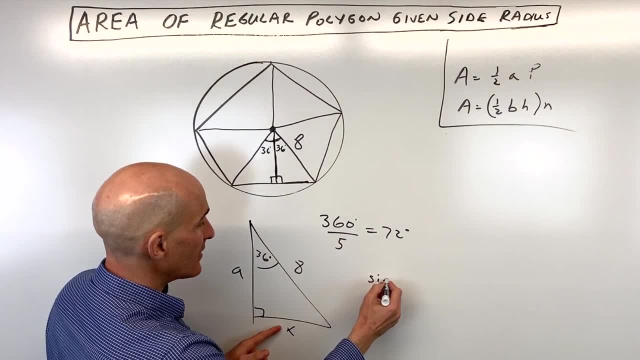 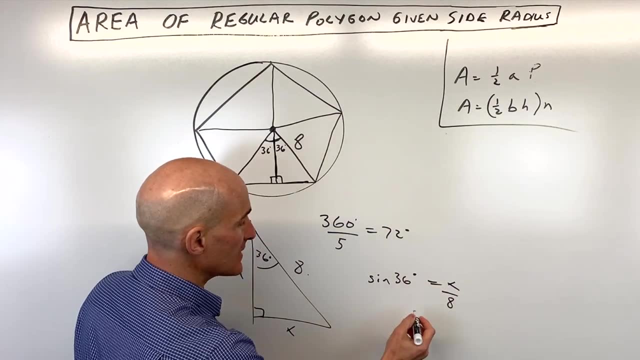 trigonometry here. Let's start off by doing the sine. So the sine of 36 degrees equals the opposite side over the hypotenuse. So that's going to equal x over eight. If we multiply both sides by eight, that's going to give us x over eight. So that's going to give us x over eight. So that's going to. 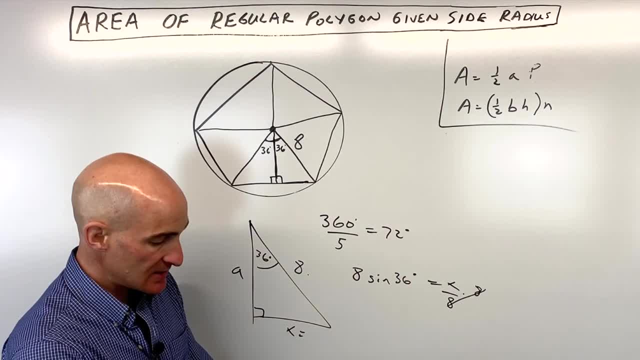 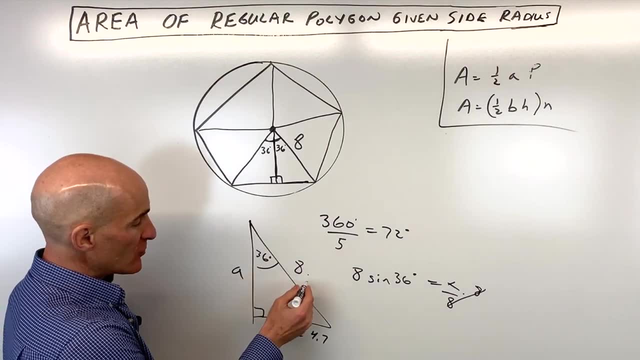 give us x here. So let's see what that comes out to. It's eight times the sine of 36.. Okay, which is about 4.7.. I'm just rounding, And then for this side we can either do the Pythagorean theorem. 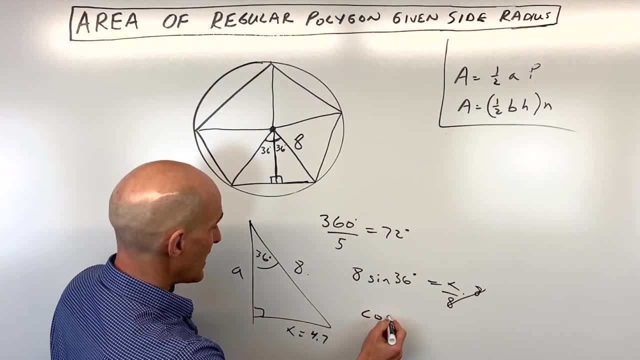 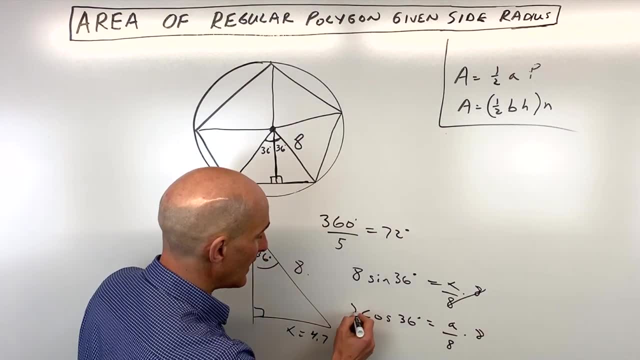 or we could do the cosine, So we could say: cosine of 36 degrees equals adjacent over hypotenuse. So that's a divided by eight. If we multiply both sides by eight, we get a by itself. So that's eight cosine 36, which is about 6.5. 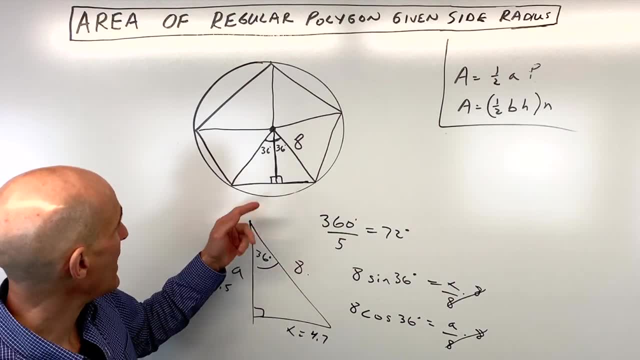 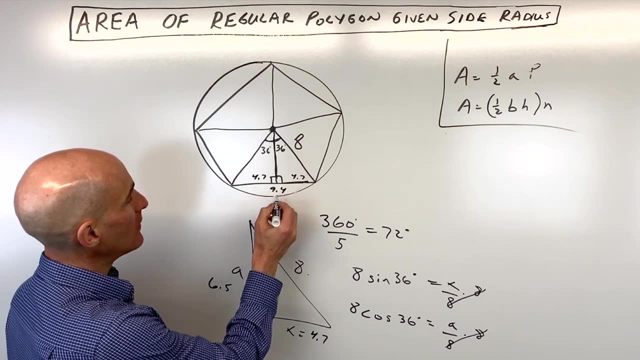 Okay, so now what we're going to do is we're going to go back to the triangle here. So this is 4.7, that's right here, 4.7.. This is also 4.7.. So that's 9.4.. And the height of the triangle we. 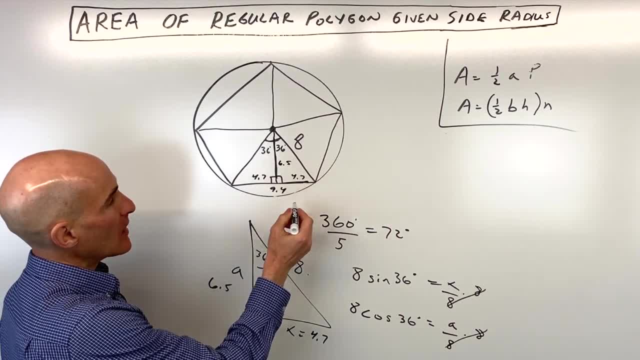 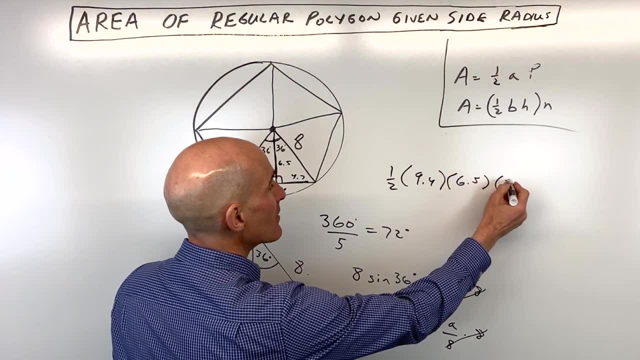 know is 6.5.. So if we want to find the area, we just have to do one half the base, which is 9.4, times the height, which is 6.5 times five of these triangles, and we've got our area. So we. have, let's see, 6.5 times 9.4.. Okay, so we know the height of the triangle is about 8.5, so we got a area. So we have, let's see, 6,, 0,, 2,, 3,, 4, and 3, so we have 6.5.. So we have six point five times nine point, four times five feet.